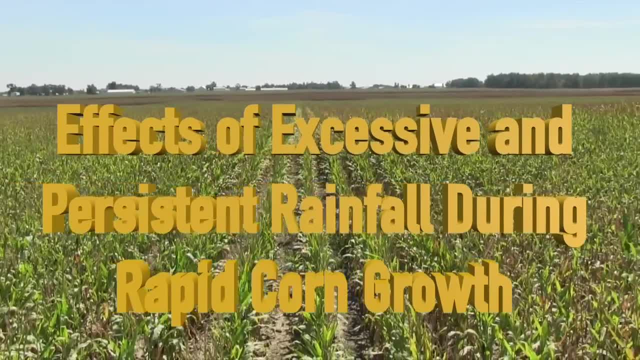 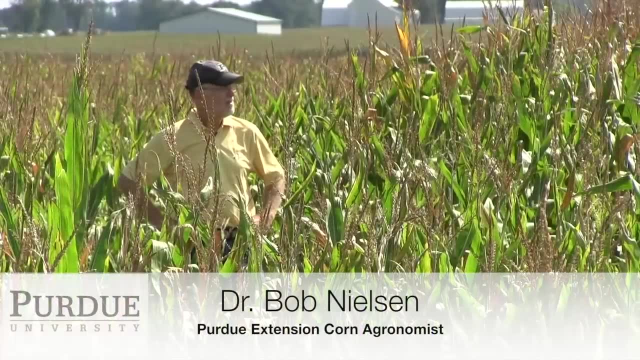 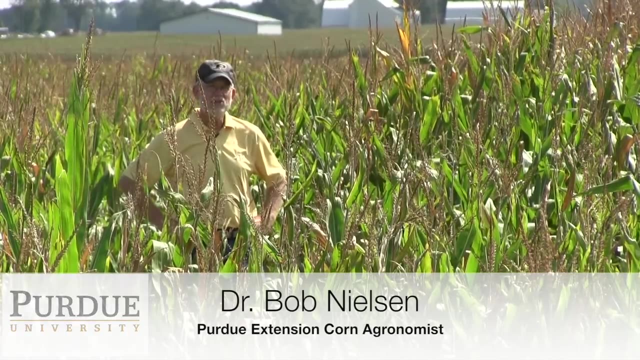 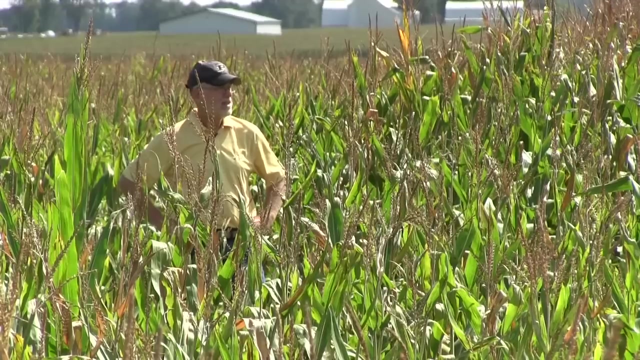 The field that I'm standing in this afternoon is an example of hundreds of fields and it's the consequence of a monsoon season, as it were, that began during planting, in some cases back in May. In other cases it started in early parts of June, But it was a monsoon. 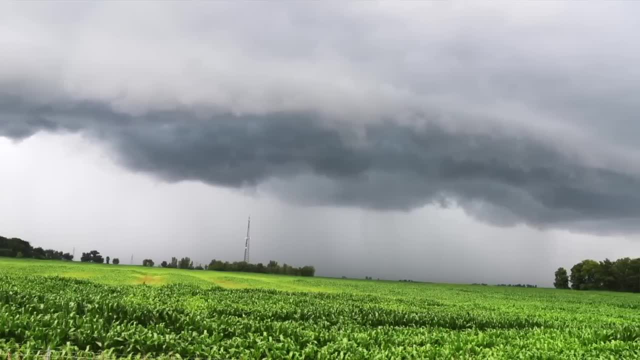 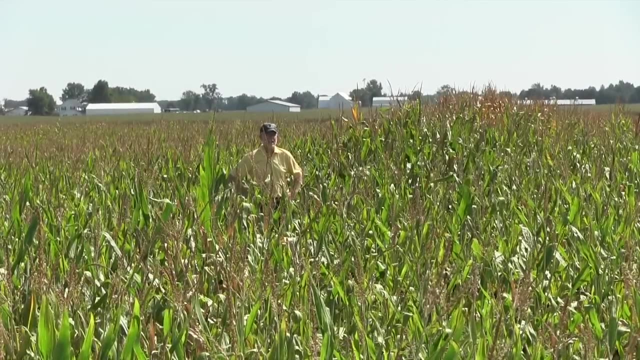 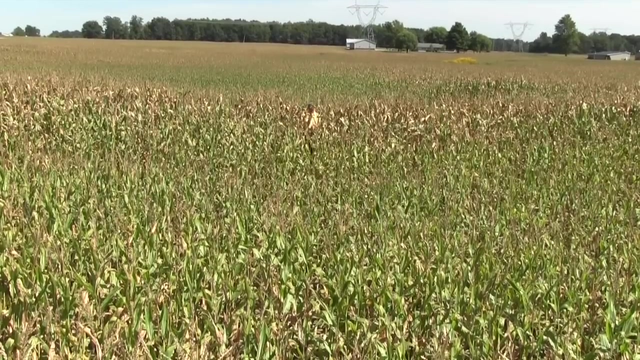 season that simply dumped untold, almost historical volumes of rainfall over a 30 day period and upwards as long as 60 days. The striking thing about this kind of excessive rainfall and the effects it has on poorly drained fields is you see the effects of the tile line where 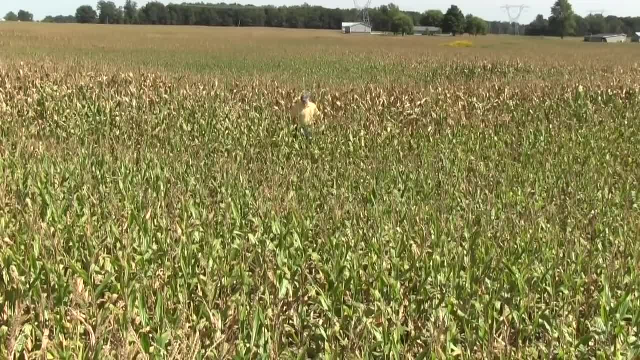 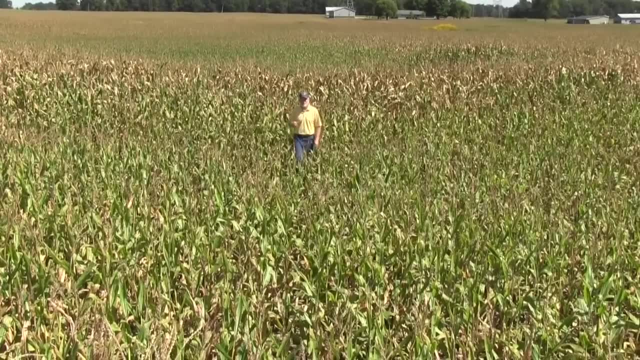 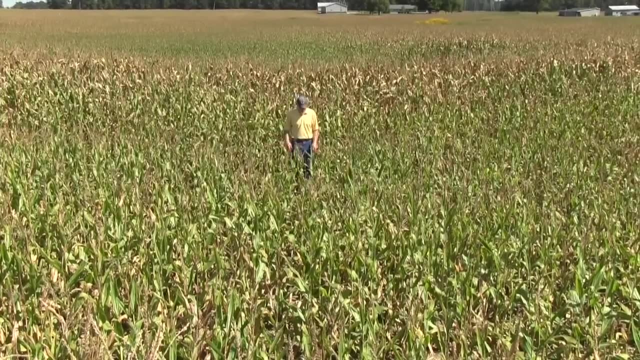 for only three, maybe four rows of corn. it's perfectly good. It's got nearly full sized ears And within such a short distance of coming off that tile line you're into this mess here which is barely waist high on me. It's got nubbins of ears or very small ears And as 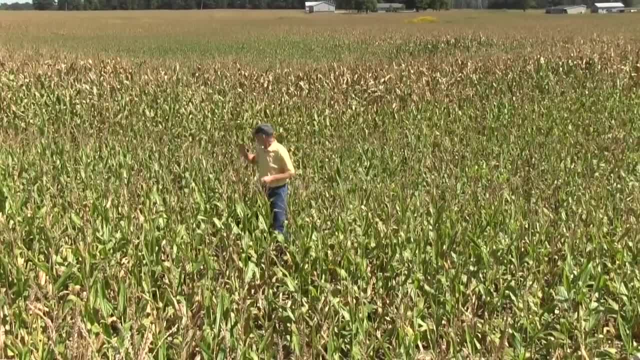 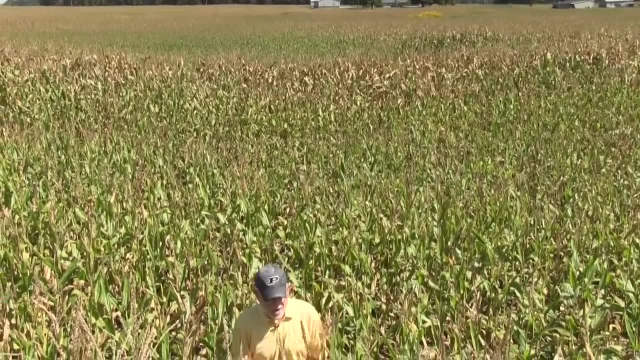 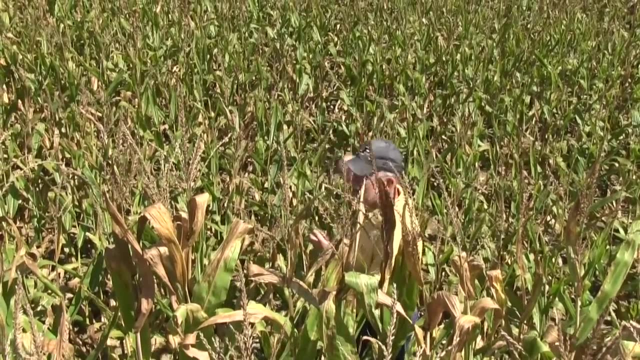 I'm walking across this. this is only about 50 feet from the tile line that I began with to the tile line that I'm coming up to, and it's just very striking what the drainage can do Now, the fact that there's such poor management of the drainage, in particular, 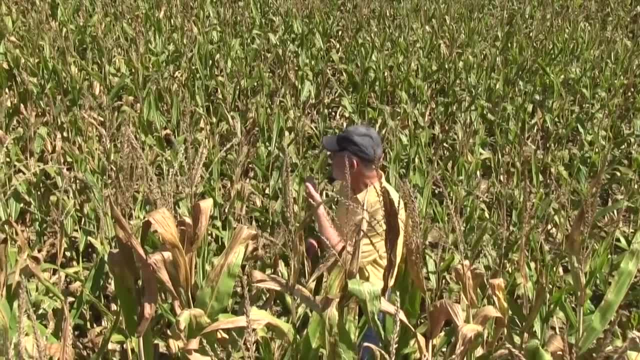 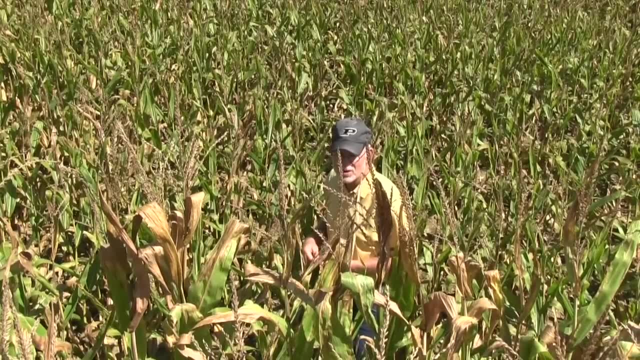 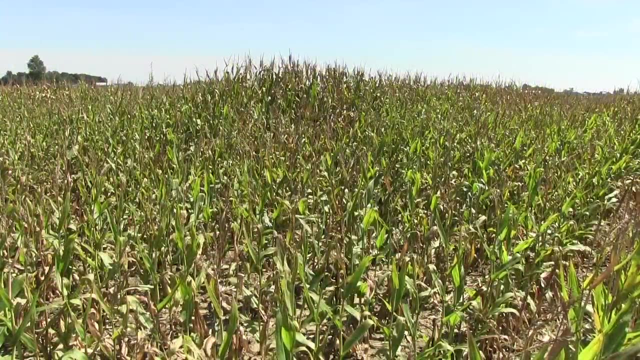 between these two tile lines is probably indicative of some historical soil compaction that's built up in this field. And it just couldn't. the drainage- or the tile drainage- just could not overcome the excessive rainfall that happened over such a short period of time. 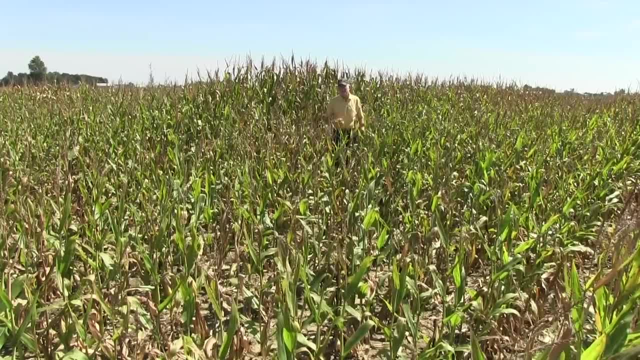 The potential in this field actually was pretty good. When you walk into these small segments of the field where it had better drainage and poor ears, you can see that there was a lot of rain that was coming from the top of the tile line and the top of the tile line. 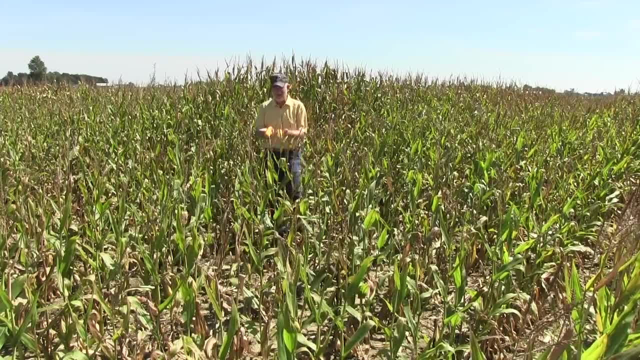 that was coming from the top of the tile line and the top of the tile line that was coming from the top of the tile line and the top of the tile line that was coming from the top of the tile line. The ears are essentially what you would expect for very good yields. 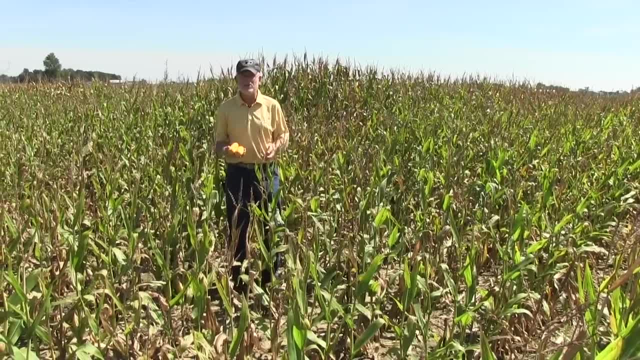 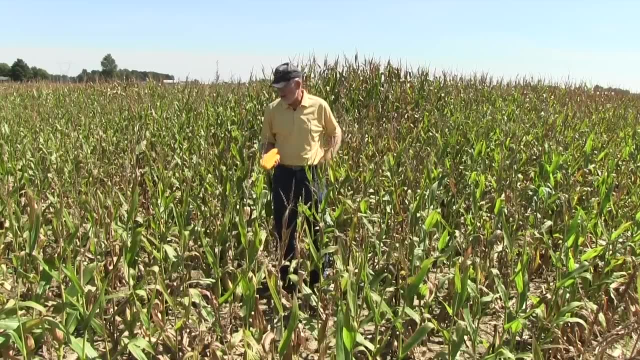 And that's why this year is so disappointing for these folks that suffer through this extensive rainfall, because when you have fields where the majority of it is as tall as what I'm standing in now and pull ears from these plants, I'll pull them out of my pocket. that's how. 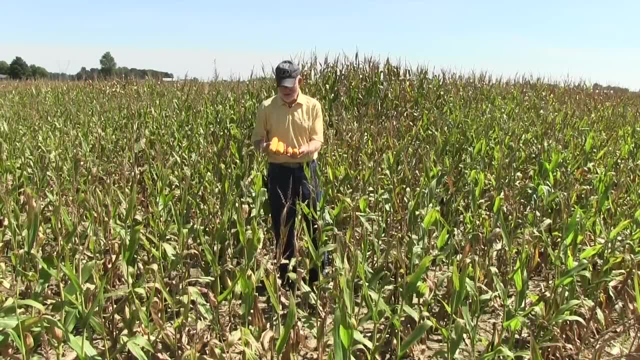 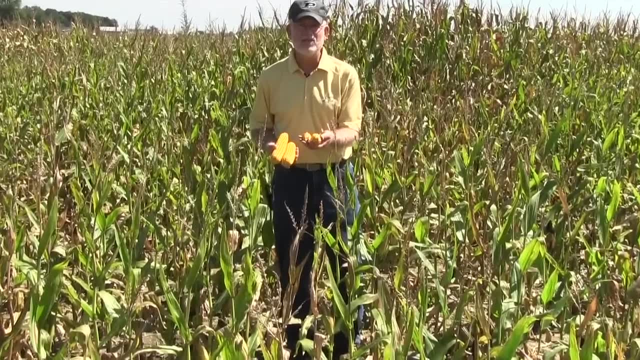 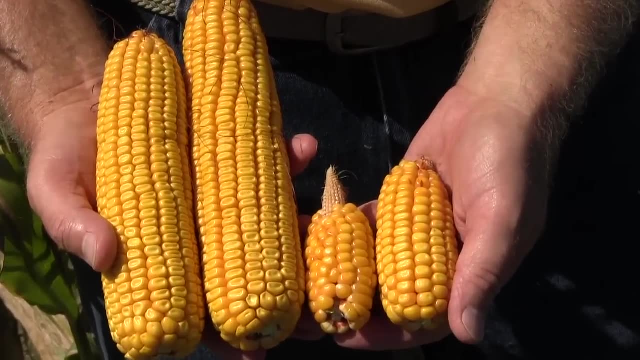 small they are. you get a world of difference on what the potential was and what the reality is. You get the kind of extensive water damage that this field endured so early in the season and it's led to these stunted plants and yield potential that is dramatically reduced. and 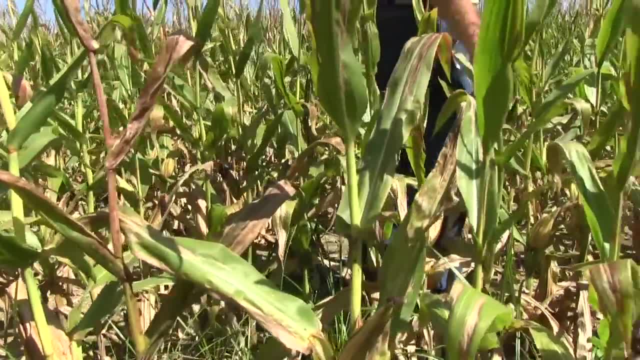 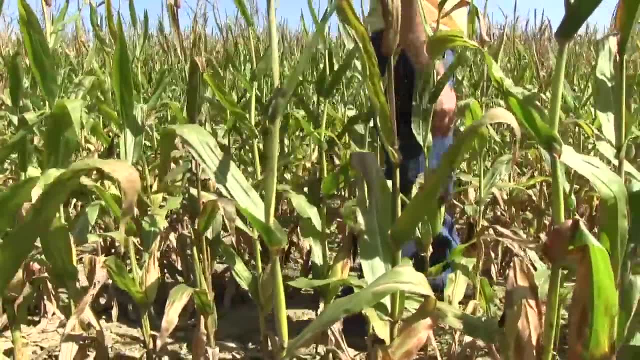 frankly, the ears on these stunted plants are positioned so close to the ground that I think in many cases the harvesting head of the combine is going to have great difficulty getting under those ears and actually getting them into the throat of the machine. So there may 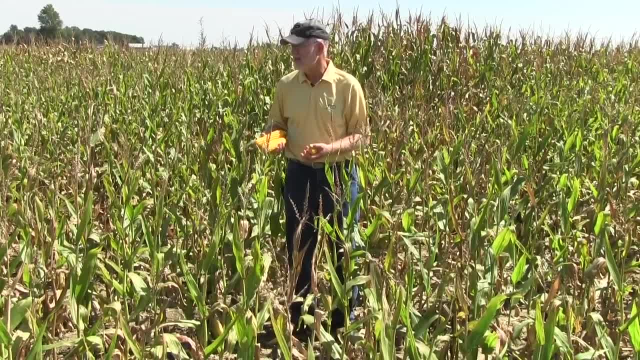 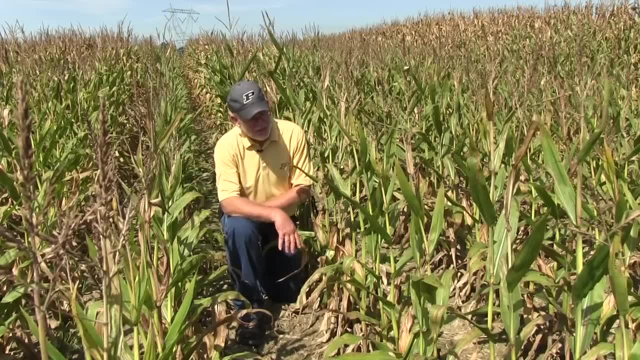 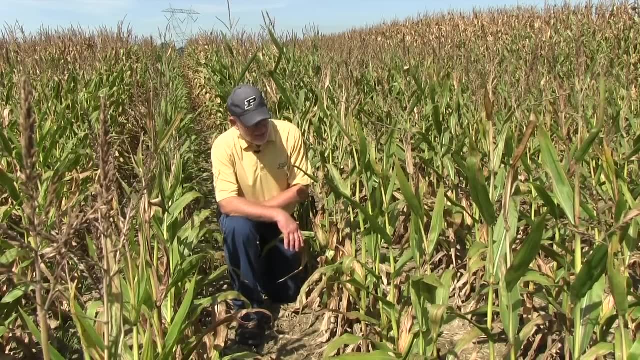 be ears like this out here, But I think in many instances the machine won't even be able to harvest it. The timing of the monsoon season, as we call it, began somewhere around the tail end of May and lasted through most of July. Well, that's clearly during almost the entire rapid. 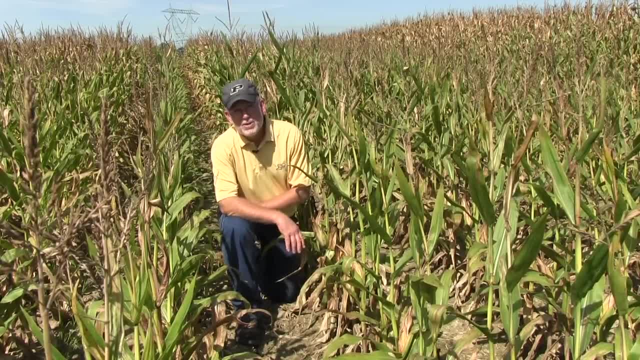 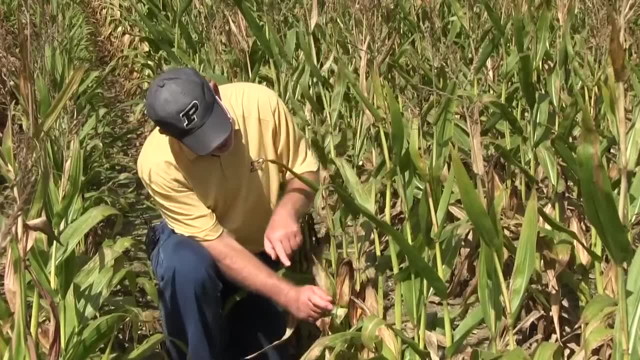 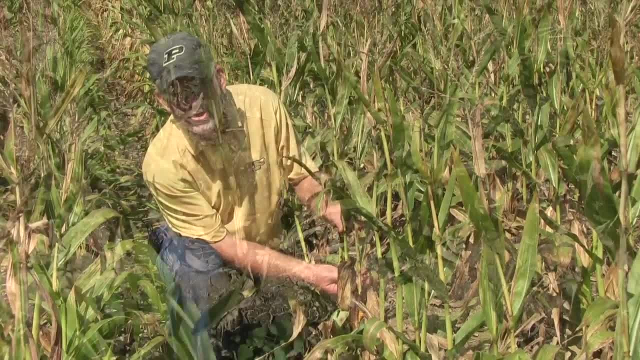 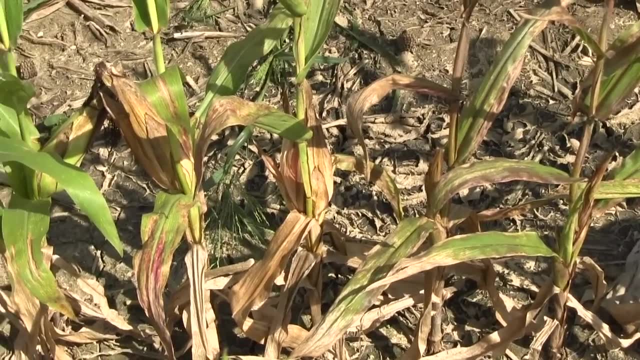 It's the space between the nodes of the stalk, and that's where the elongation occurs. When there's that much stress imposed on the plant, photosynthesis is not working correctly and nothing is functioning very well. This elongation process is stunted and that's 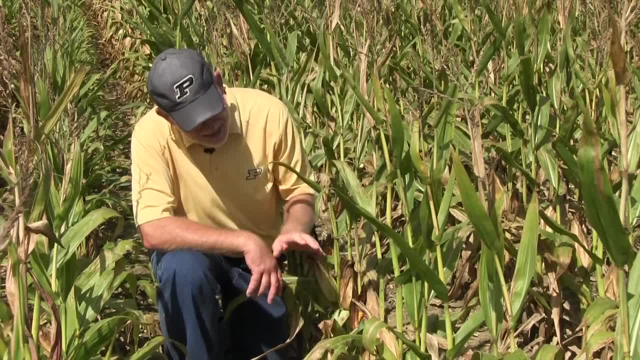 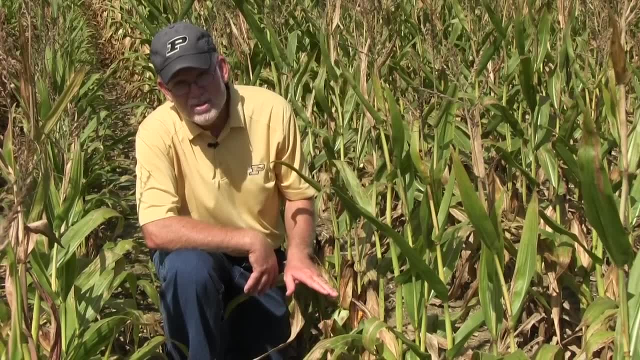 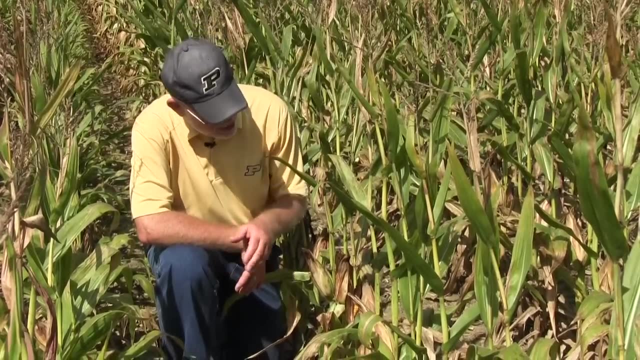 why, then, in such an early timing of stress? that's why these ears now are positioned so close to the ground. It's not that they're positioned at different nodes than they normally would. It's the fact that these internodes below them were stunted so severely during the elongation process that the natural node of this plant. 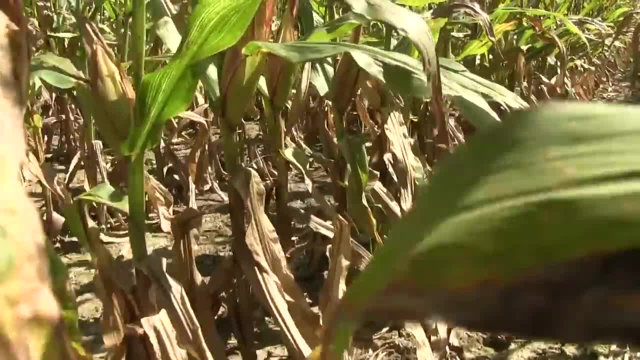 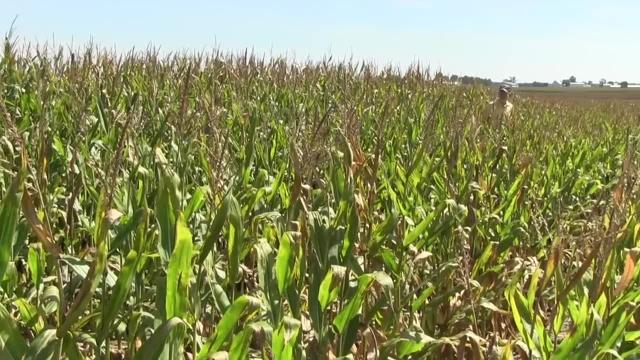 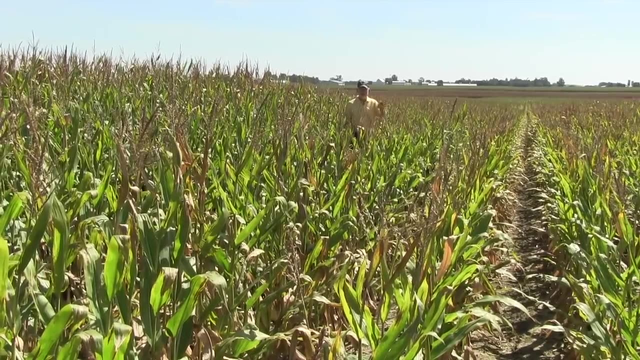 is now only about 18 inches, or say knee, high above the ground. When there's this much difference in height of the plants, I would have expected that there would have been a real strong delay in the development of this stunted corn, And because of that I really expected that the kernel development on the ears would be. 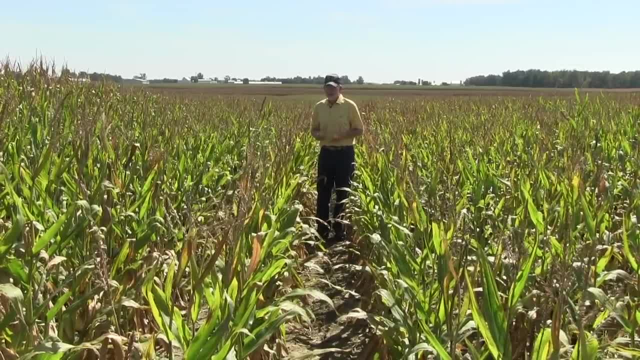 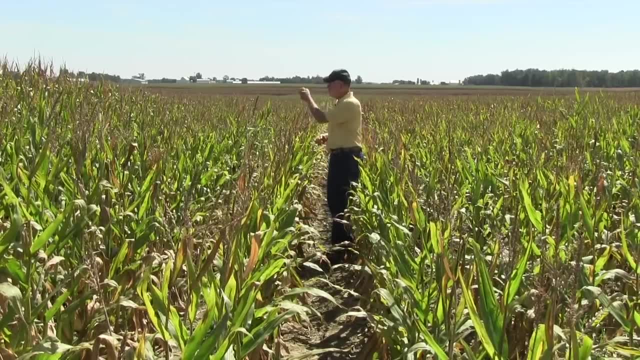 much farther behind And if that were true, I was thinking that we would be seeing a lot of difference in grain moisture at harvest time. But, interestingly, the good ears that I pulled out of that tile line and the ears that I pulled out of the stunted- interestingly. 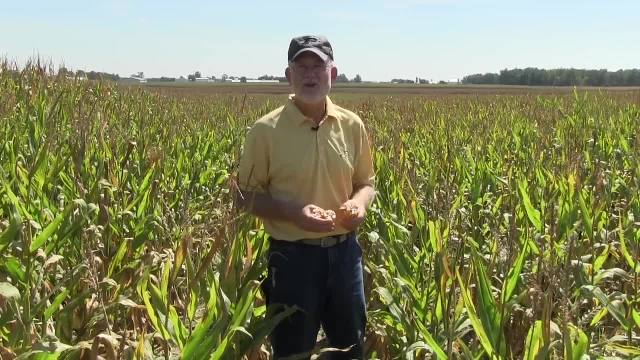 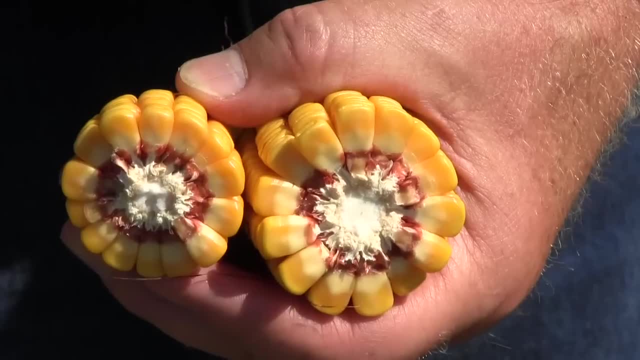 there's very little difference in the progression of the milk line on the face of the kernel. The ear on this side came from one of these stunted plants. The larger ear came from the plants over the tile line that are much taller and healthier. 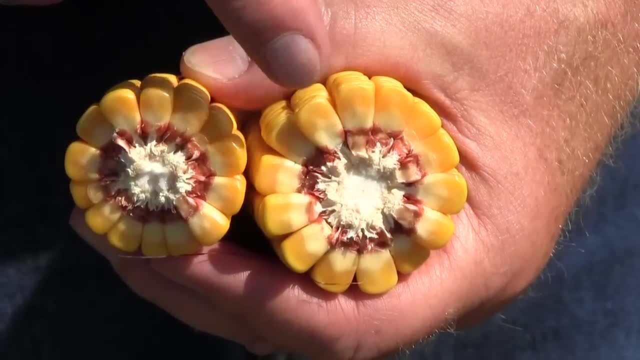 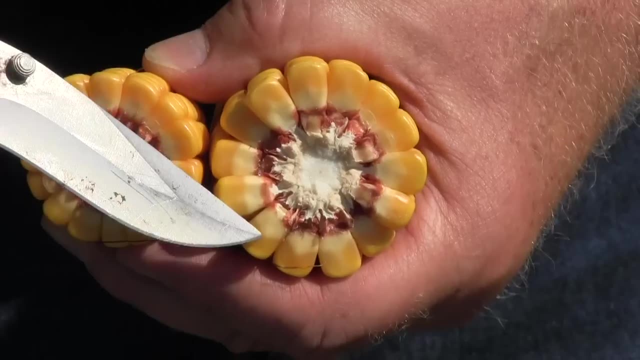 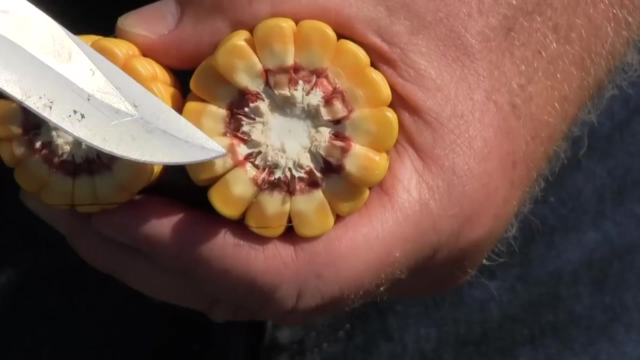 And I would have expected that the better ear would have been farther along. But at this point in the grain fill process what we're looking for is this sort of imaginary line between the darker, drier starch near the tip of the kernel and the lighter colored. 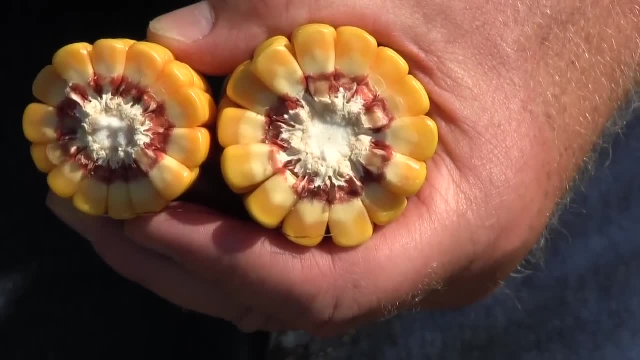 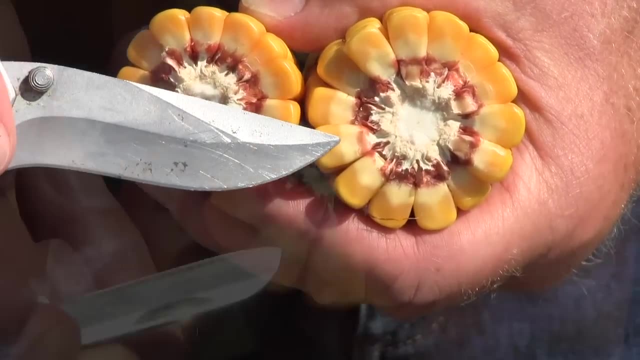 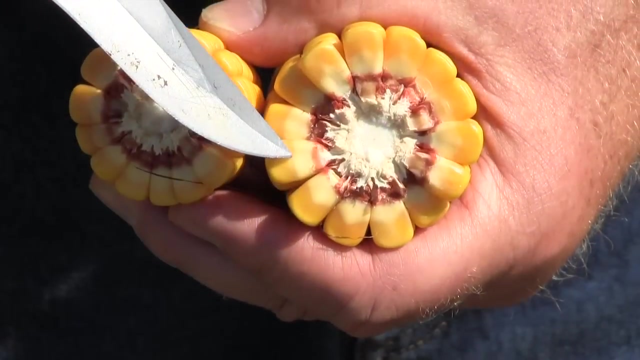 and still liquid part of the kernel down near the cob, And this interface is called the milk line And on both of these the milk line is about, oh, half the way down from the crown of the plant And, of course, as these ears get closer to maturity, this milk line progresses. 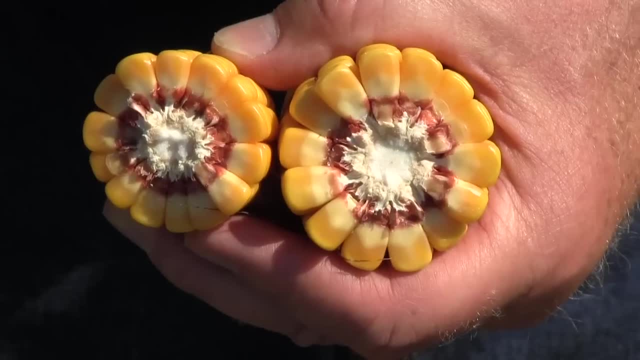 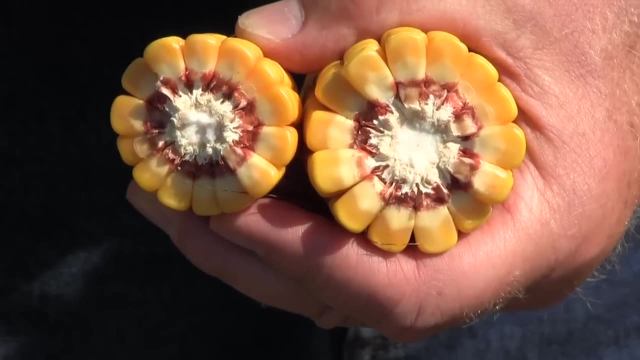 all the way down and eventually disappears into the tip of the kernel. And yet both of these ears seem to be at approximately the same stage of development. So if that's true, then in this field at least, there would be very little difference in grain moisture in. 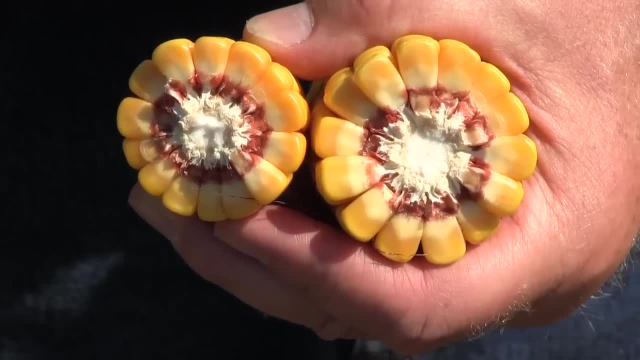 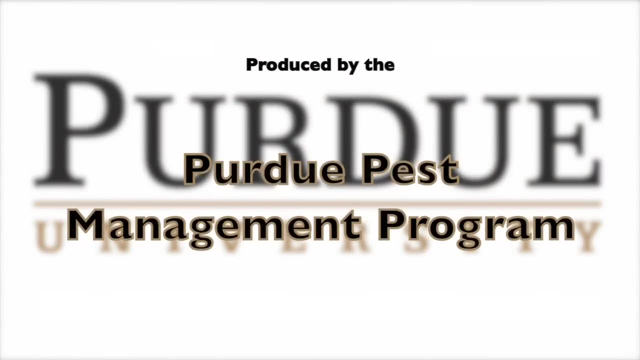 the grain harvested from the stunted areas compared to the grain harvested over these better drained areas of the field. Subtitles by the Amaraorg community.